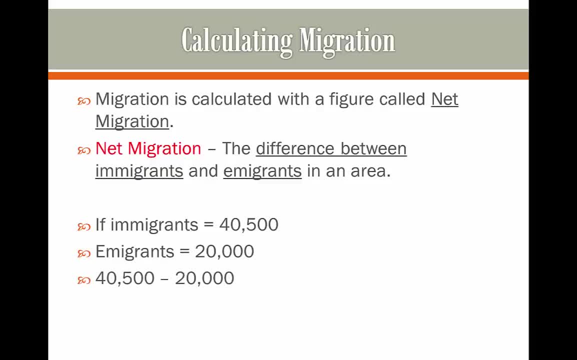 two figures. So we subtract 20,000 from 40,500 to get a net migration total of to 20,500.. So this is a positive migration Because there are going to be more immigrants coming into the country. then there are emigrants. 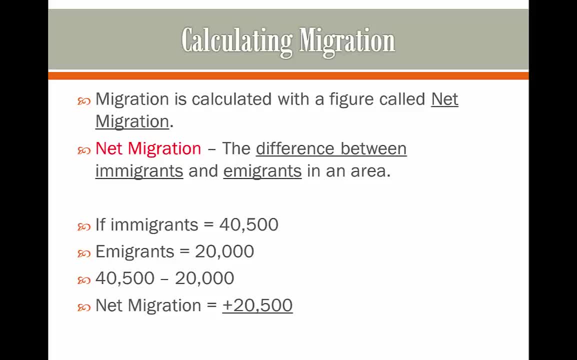 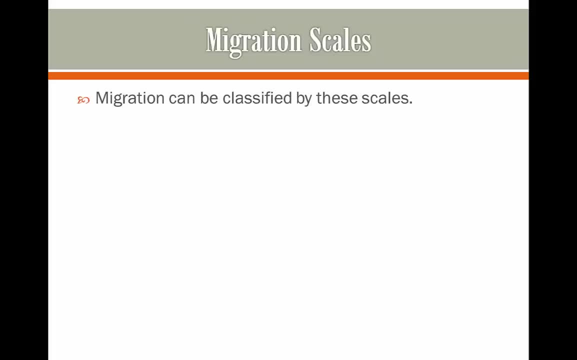 leaving the country. If these figures were inverse, then we'd have more emigrants than immigrants and there would be a negative balance. Migration scales: Migration can be classified by these different scales Where people migrate, So it can either be international, regional or local. 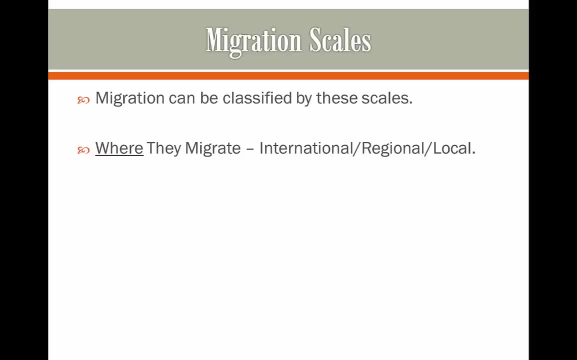 Remember in the definition of migration is a permanent or semi-permanent change in residence. So it doesn't necessarily mean that people are going to be leaving the country, So it doesn't mean having to cross a border. You can simply migrate from one town to perhaps a town in another. 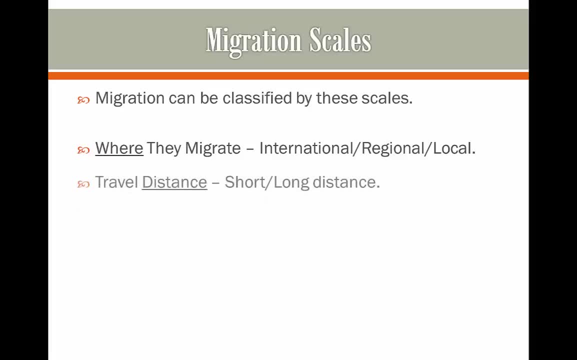 city and that would still be classed as migration. The travel distance, So it can either be short or long distance. Travelling from one town to another may be deemed as short distance, But travelling from Poland to the UK in order to look for a job is a long distance migration route And the time 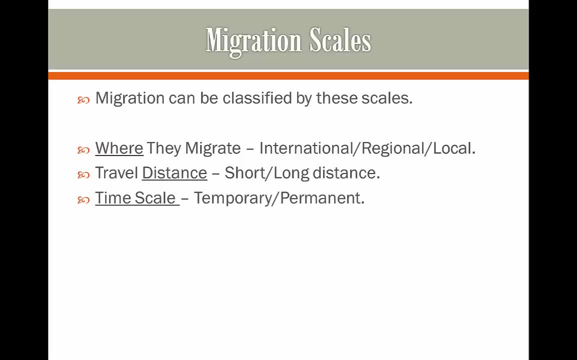 scale. As we know, migration can be semi-permanent or permanent, So it doesn't necessarily mean that people are going to be leaving the country. So it can either be a temporary placement, For example, going abroad for one year of work, or a permanent placement, But either way you are migrating. 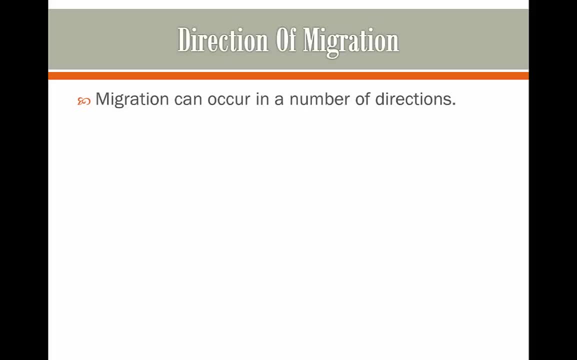 Direction of migration. Migration can occur in a number of directions. It can be urban-rural or rural-urban. What this means is that you're travelling from a more developed urban area to a less developed rural area, or travelling from a less developed rural area to a more 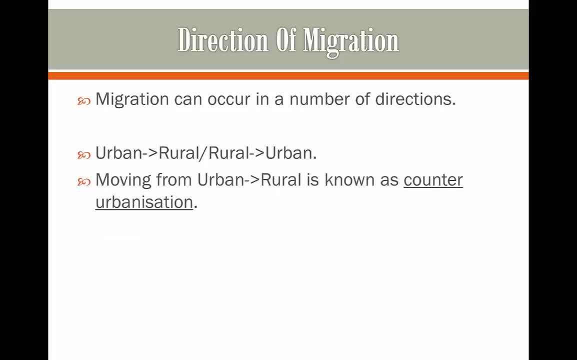 developed urban area. Travelling from an urban area to a rural area is known as counter-urbanisation. You can also travel from a developed to a developing or developing to a developed country. For example, if we were to travel from the UK to an African country, the likelihood is this would be a developed country. 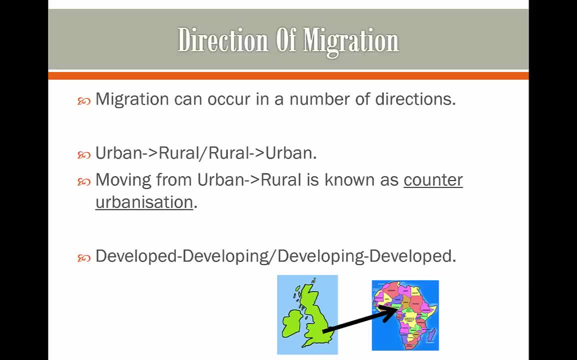 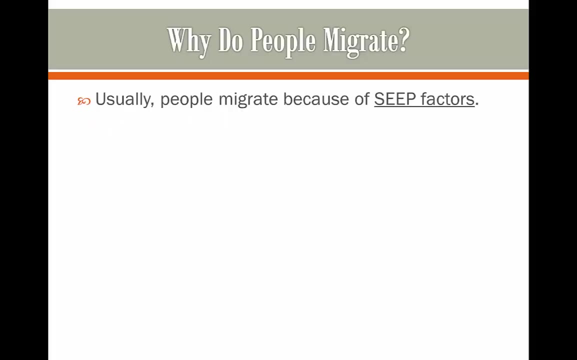 moving to a developing country And, seeing as we're probably moving from London to a remote area in Africa, it would be urban-rural, So we would be doing counter-urbanisation. Why do people migrate? Usually people migrate because of work, and this is pretty much covered.